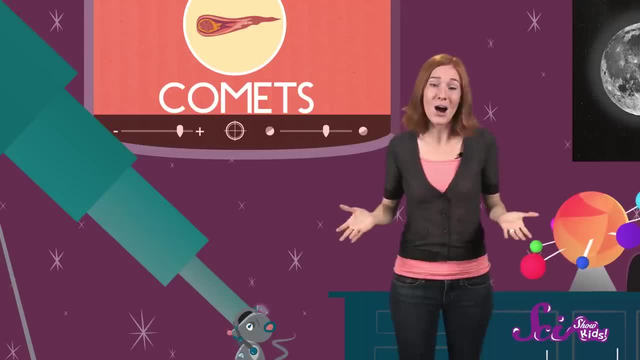 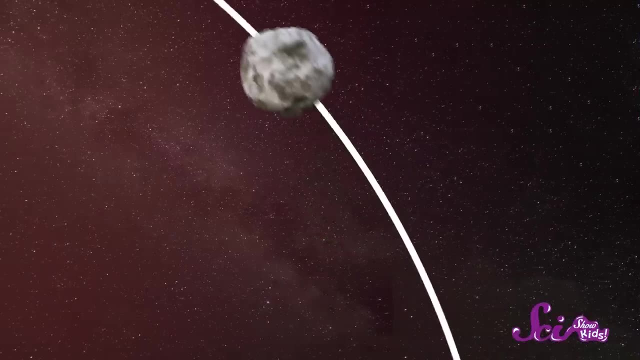 to comets as hairy stars. But why? A comet isn't a star at all and it doesn't have hair. It's really a chunk of ice, dust and rock. Think of it as like a big dirty snowball in orbit around the Sun. 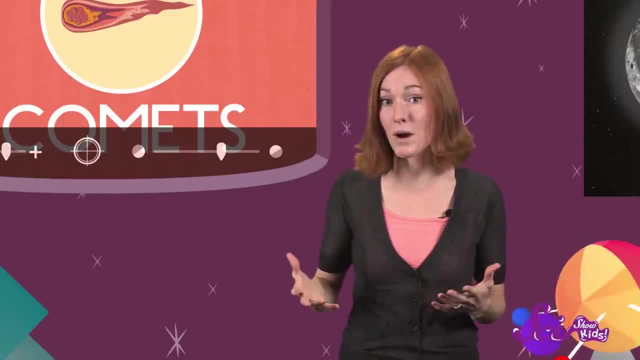 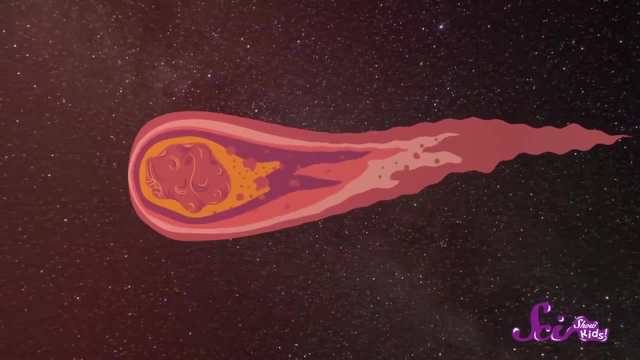 As a comet gets closer to the Sun, its frozen gases and dust begin to warm up and thaw out. The gas and dust start to break apart and stream behind the comet, making it look like it has well a big, hairy tail. Our solar system's most famous comet is probably the one known as Halley's Comet. It's named after English astronomer Edmund Halley. Halley figured out what it really was. He had read reports about three comets that were seen flying by the Earth many years apart, But Halley figured out that these three comets were actually the same comet flying past. 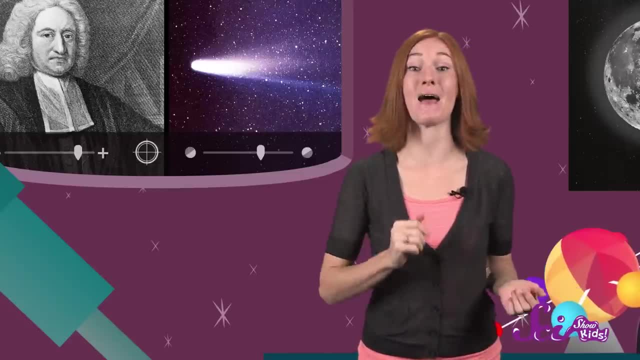 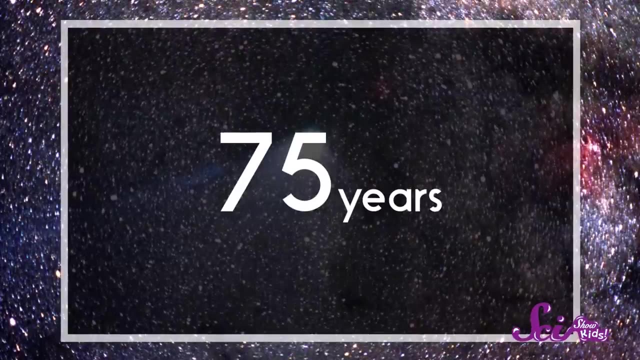 us over and over again. Based on when the comet had passed by the Earth in the past, he predicted when it would come by again, And he was right. Halley's comet has been spotted from Earth every 75 years or so. The last time it came close was 1986, meaning we'll probably see it again in 2061. 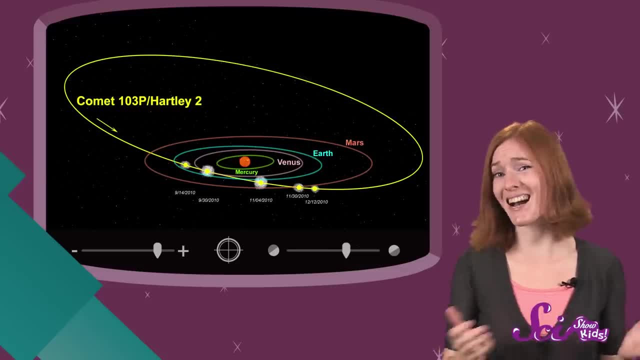 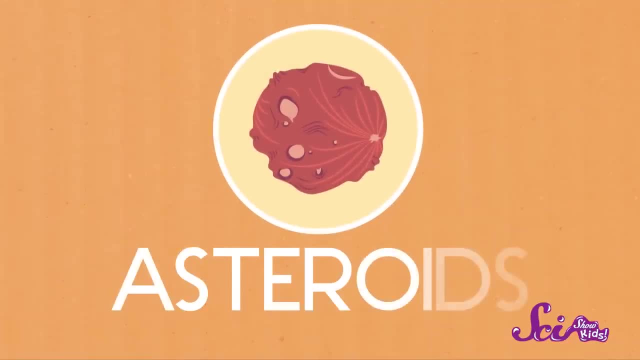 How old will you be then? Now, comets have really big orbits. They take a lot of their time in the far outer reaches of our solar system, So let's talk about rocks that come a little closer to the Earth — asteroids. 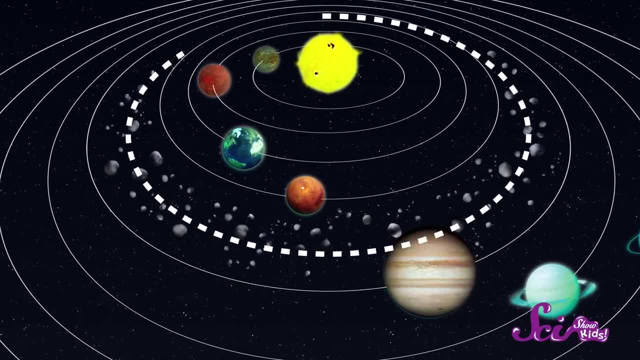 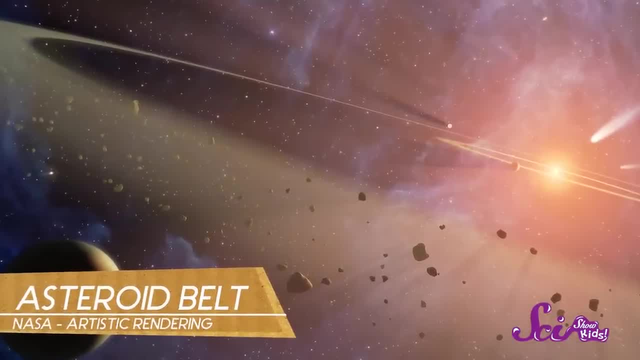 Most asteroids are found between the planets Mars and Jupiter in an area called the asteroid belt. There are a lot of asteroids cruising around in the asteroid belt, but most of them are spaced really really far apart. Asteroids sort of look like comets, but they don't have fuzzy outlines or tails. 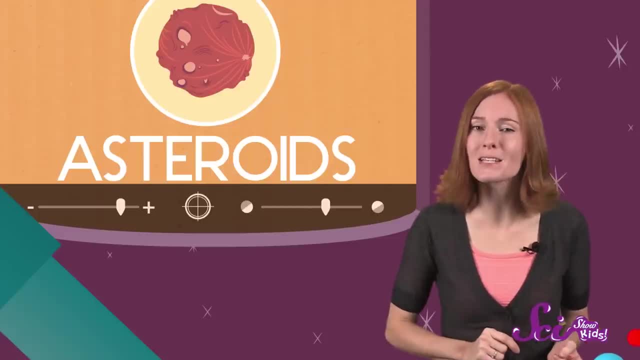 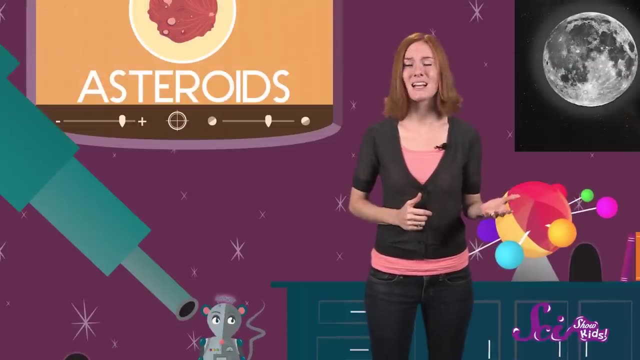 Actually, they look a lot more like tiny planets. In fact, one famous asteroid named Ida even has its own moon. It's called Dactyl. Asteroids are basically broken pieces of unfinished planets left over from the time when the solar 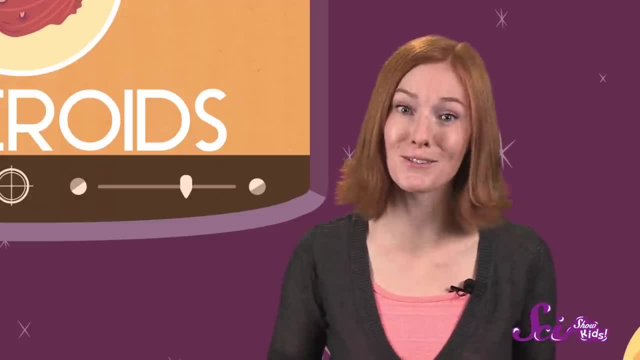 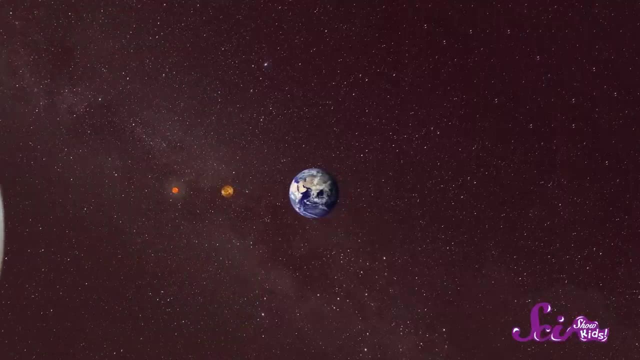 system first formed. They're mostly big chunks of rock with metals in them too, And as they fly around out there in the asteroid belt they often crash into each other. Sometimes an asteroid will get bumped clear out of the asteroid belt. 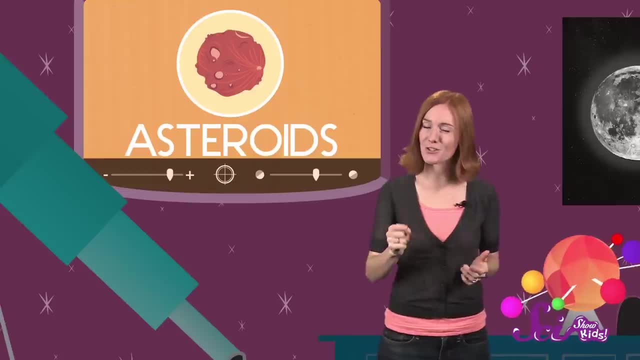 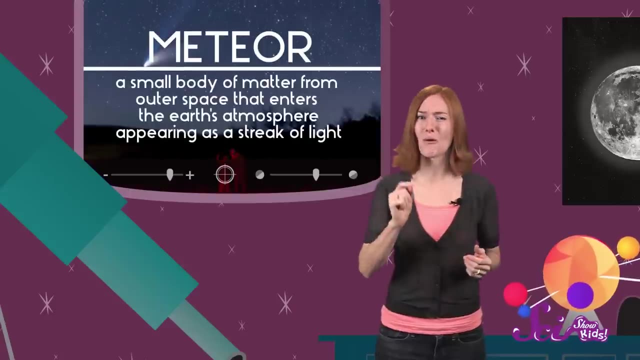 They can even get knocked in our direction. If a flying space rock enters the Earth's atmosphere, which is what we call the layer of gases that surround our planet, it'll start to burn up. Then it's called a meteor, a really fast streak of light that flies through the atmosphere. 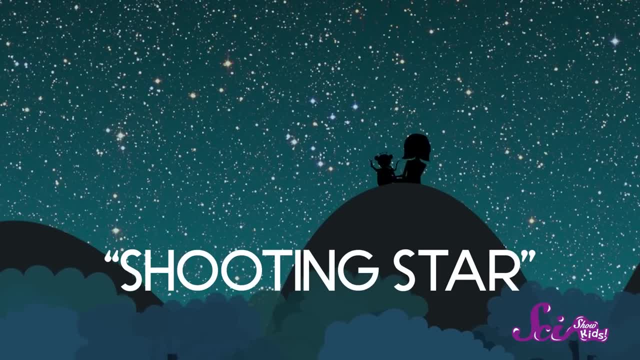 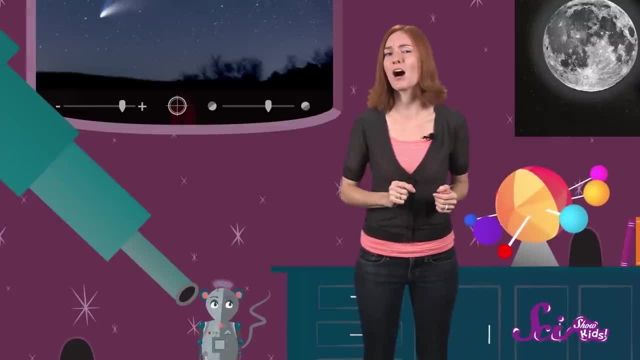 You might have heard this called a shooting star, but now you know it's not a star at all. Most meteors burn up completely before they reach the surface of the Earth, but if a hunk of rock is big enough, then some of it might still be left by the time it reaches the ground.